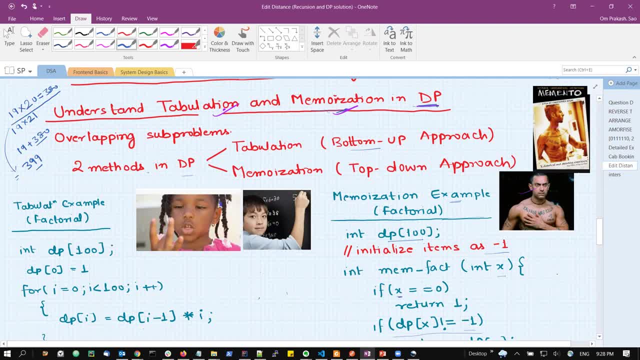 Now, this reusing of the same sub-problems can occur in two ways. One is tabulation, One is memoization. If we will go by definition, tabulation is basically following the bottom-up approach for saving the result of sub-problems and reusing them. 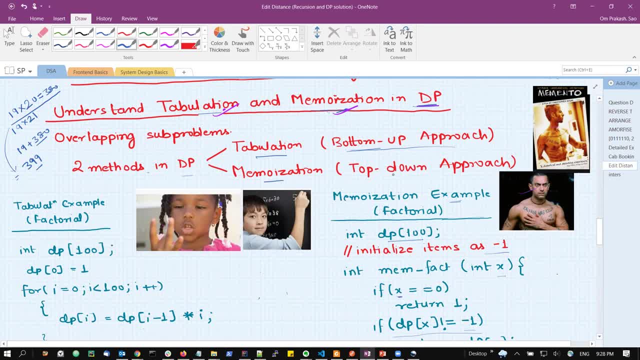 In the same way, memoization is top-down approach for the same procedure. Let's say that: what is tabulation, What is tabulation? So when I was studying this topic for the first time, I was getting a little bit confused that what is the difference between them? 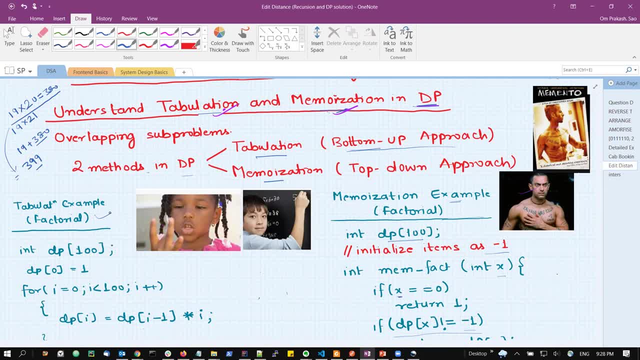 So I will just explain it to you using one example. So what is tabulation? So in tabulation let's imagine there is a child who knows only the addition. He doesn't know that what is the multiplication? So if we ask him, what is 5 into 9?? 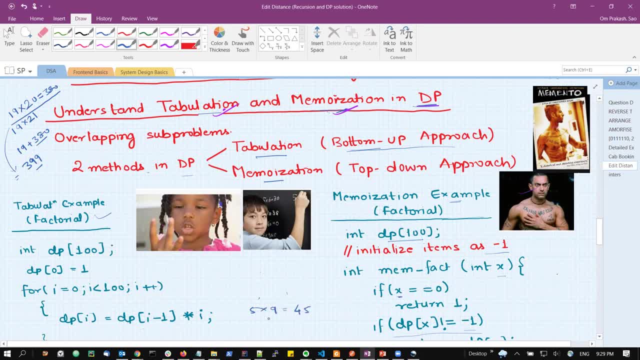 So it is 45. But he doesn't know it because he doesn't know what is multiplication concept. So what he does is he starts counting the multiplication table: that 5 into 1 is 5.. 5 into 2 is 10.. 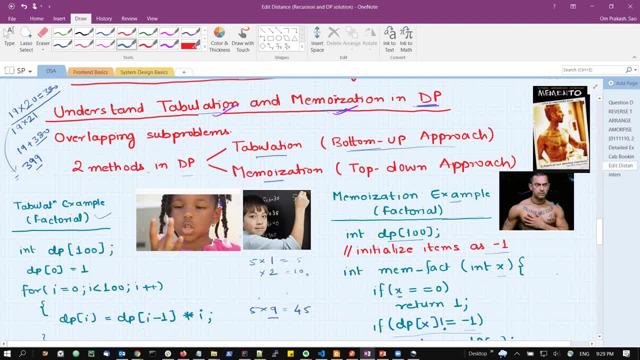 So basically, what he is doing is he is adding 5 each time to the previous result, So he is creating a kind of multiplication table to arrive at the solution of 5 into 9 is equal to 45.. So this method of starting from the most smallest sub-problem and going one step up, one by one, 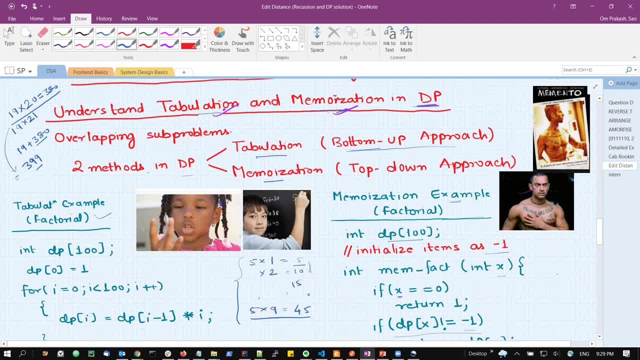 This process is called tabulation, So we can just remember it that tabulation is the process how a multiplication table is built. So tabulation and multiplication table. We can remember it like that. Tabulation is a bottom-up approach. Now let's come back to the memorization. 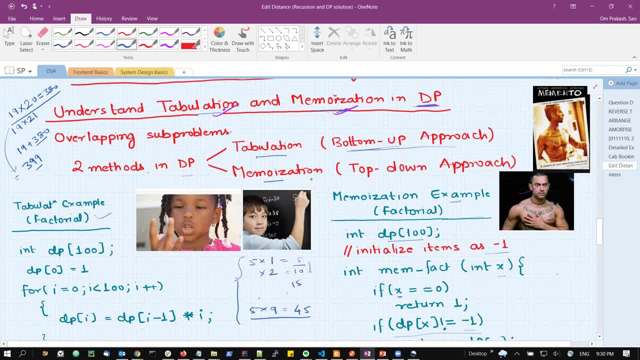 So let's see, there is one funny example of there was one movie, Hollywood movie, Momento, And the Bollywood remake of that is Gajni. So in that movie the actor has a forgetful personality, Where he forgets that. what's going on? what is the current situation? 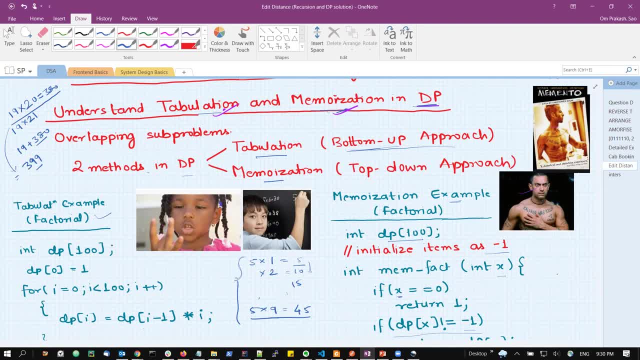 So, in order to remember the past, he wrote or he tattooed the important events of his life. So let us say there is an actor and he has written some of the important events, But he doesn't remember those events. So what he will do, 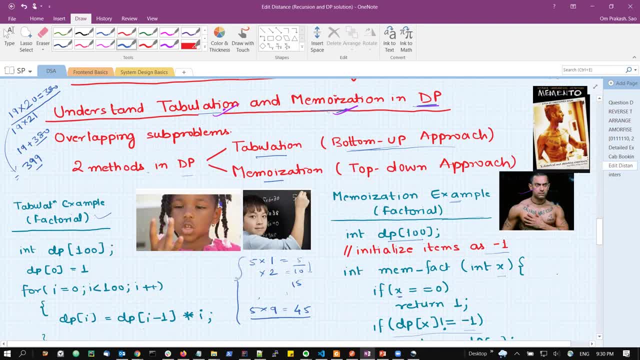 He will, let us say he wishes to remember something which he has encountered. So, in order to remember that, he will start looking for that particular tattoo in his body. But in those process he will find some other tattoo And now he will start looking for the information about that tattoo. 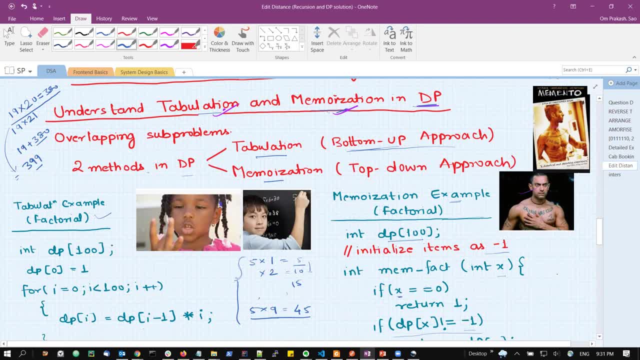 So it is kind of a recursive call, one by one. He will keep looking at the tattoo, which will come on the way till he finds the answer of what actually he was looking for. So top-down approach is the same Where we are looking for a particular solution. 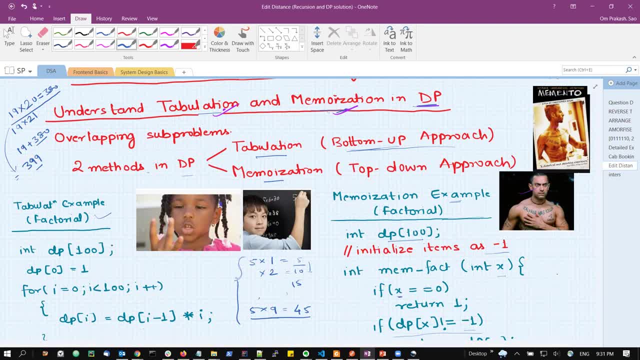 A problem's solution. But in order to find that solution, we will start breaking it one by one, At one level, by one level, And we obviously don't know the answer of one level below, So we will go one level further below. 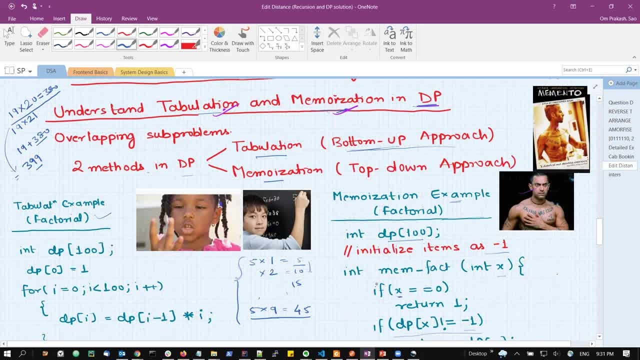 Till the point we know the answer. So it is kind of a recursive call in a top-down approach. Let us understand is we will start it using a proper example of factorial. So we all know what is factorial right. Factorial of any number is basically multiplying one into two, into three. 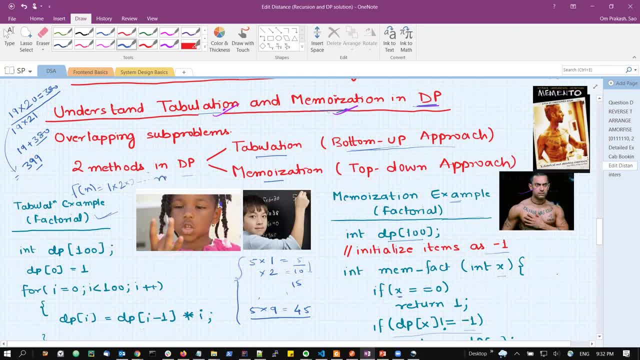 All the numbers till that number n, That is factorial of a number. Okay, Factorial of zero is one, And factorial of one is also one. They are generally taken as a base case. So if we have to calculate factorial of 100,. 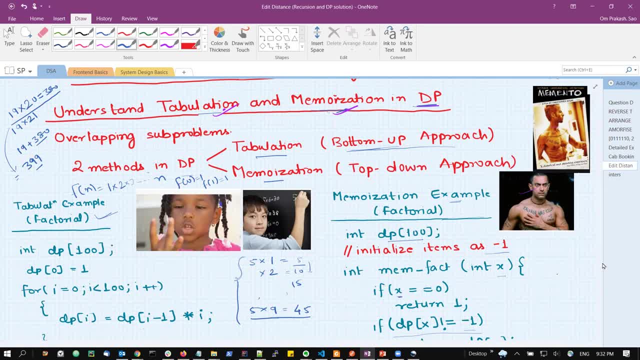 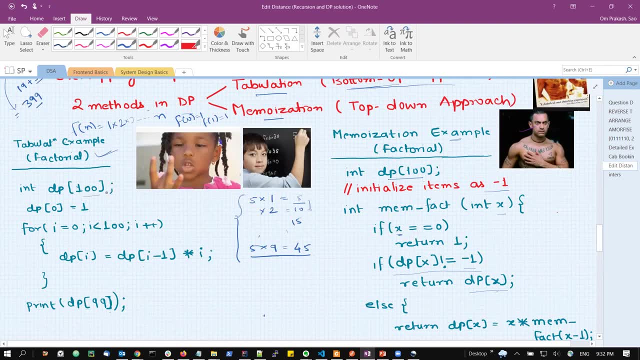 using tabulation method. let us say So. what will happen is: yeah, What will happen is: we will create an array of 100 sides. We will initialize the first, first index or the first element of the array as one, Because the 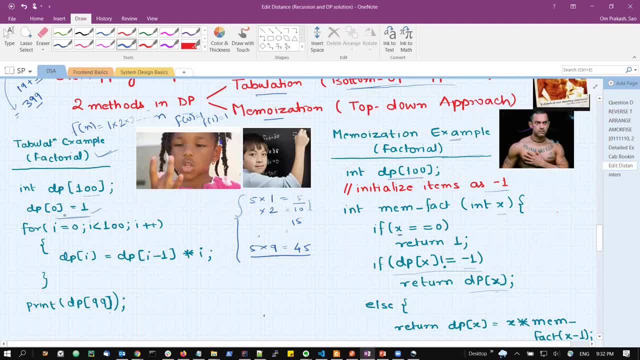 the, the factorial of one is one. Okay, And now we will start from. i is equal to zero, Basically the first factorial to the hundred factorial. So basically we are storing the factorial one at the index zero, factorial two at index one, and so on. 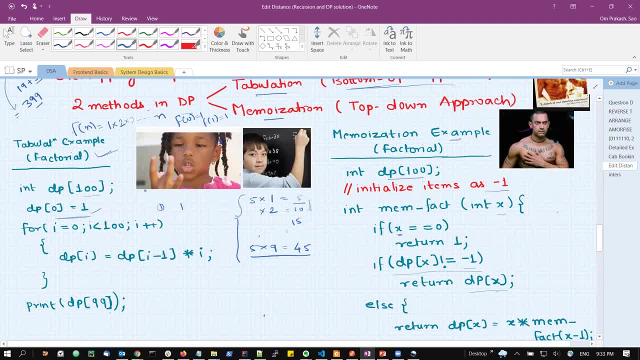 Okay, Just remember that, because the array representation is zero, index or zero based. Okay, So now, whenever we are going one level up, for example, factorial of one is zero, factorial of two is stored in the index one, which is one. 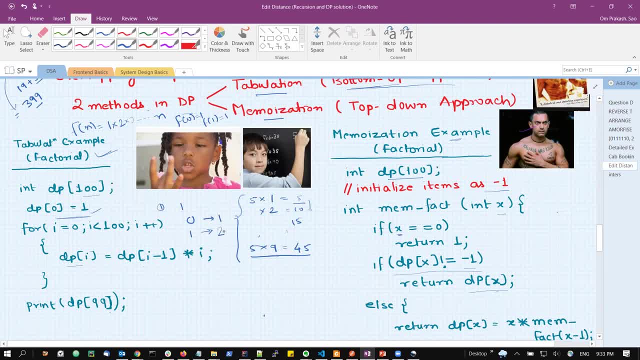 One into two, So it will be two, and so on. So in order to calculate the factorial of i-th index, we will multiply it with i and the previous element. So in this way, one by one, one by one, we are going to calculate each of the factorial. 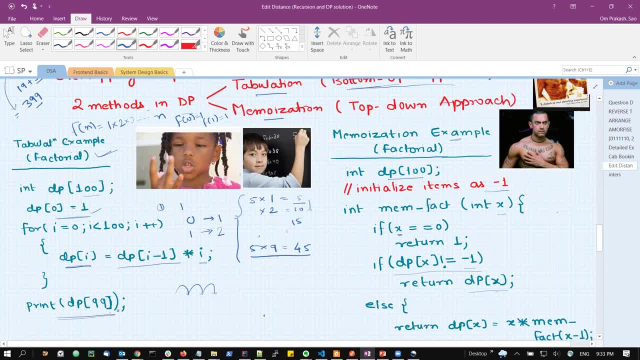 At the end, all our elements, all the elements of the array, will have the factorial for the corresponding values And we will just print factorial 100 as dp 99th index. So this is a way. this is a very simple example. 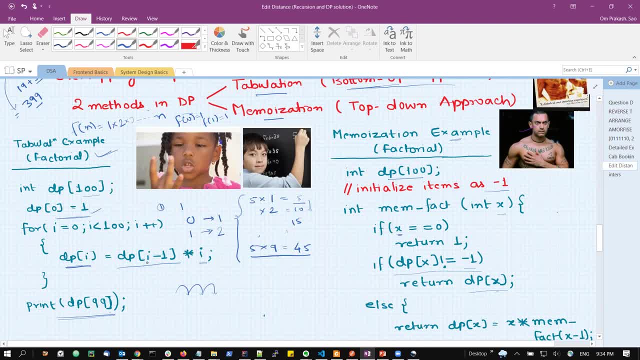 It is not a very accurate example, because this is not a not a perfect solution, a perfect, you know, way of solving the problem of factorial, because here there is no point in storing all the numbers when we just need the previous number. 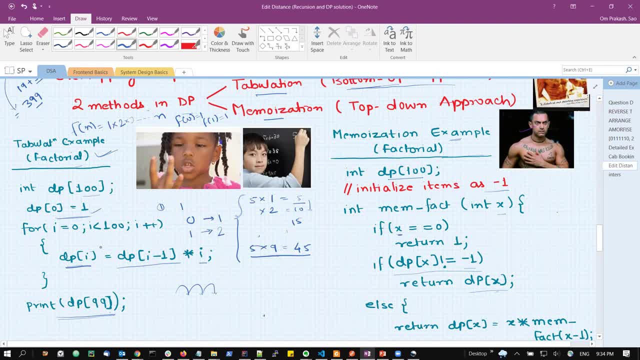 Right. So for an example of tabulation, this works fine. Okay, So this is how tabulation work. We start from the most simplest or most smallest problem and we make our way to the required solution one by one in a bottom up approach. 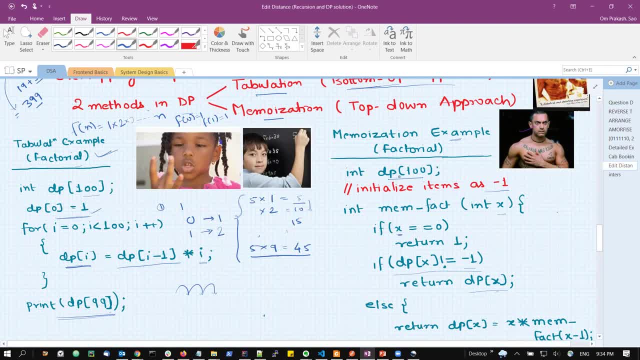 Okay, What is memoization? Let us come to this. So, in memoization again, let us say that we are looking at the same example of factorial calculation, for the n is equal to 100.. We have an array. We initialize all the element as minus one. 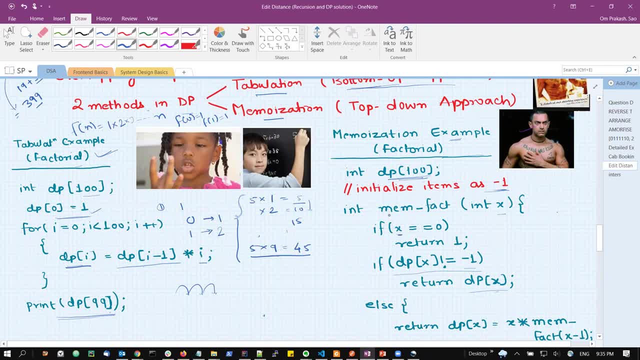 Okay, We initialize all the element as minus one and we write a recursive function- memoization factorial- which takes an argument x If x or the index is equal to zero. we know that the factorial of one is one, So we will return one. 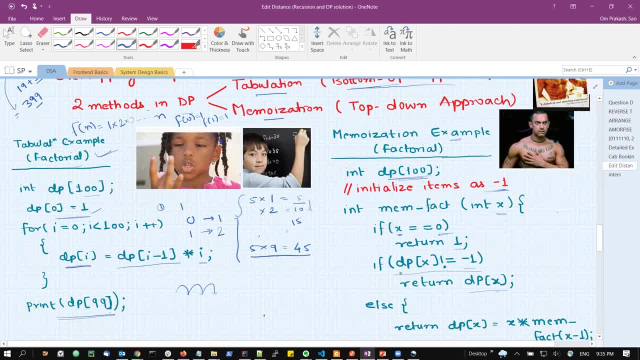 We have initialized all the elements as minus one. So if, let us say, if we encounter any index and that index, the element for that index is not equal to minus one, it means that we have calculated that particular element. So in that case, 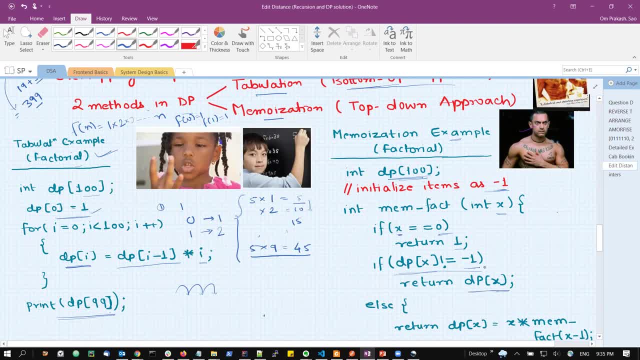 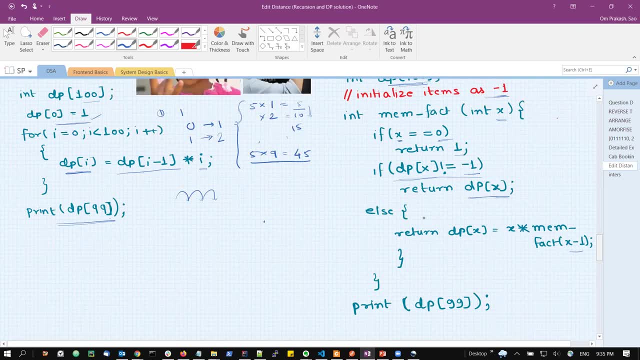 we will return that element because it is not minus one. It is some value. There's some correct value, Okay. Otherwise, otherwise, when it is minus one, okay, this is, if so, else will be minus one, right. So in that case, 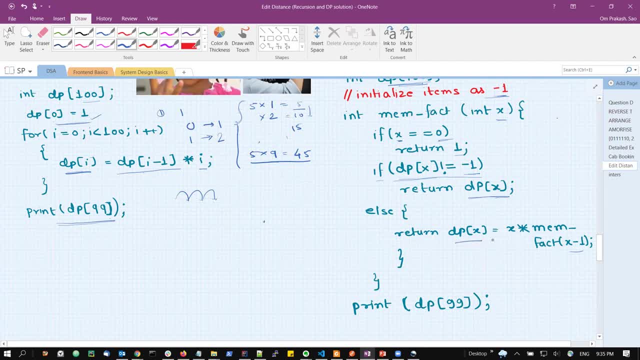 we need to calculate what is the factorial of that number. So we will use x into we will call again the factorial of one lesser number. Okay, So in this way it will make recursive call, For example, factorial of hundred. we'll just check: is hundred equal to equal to zero? 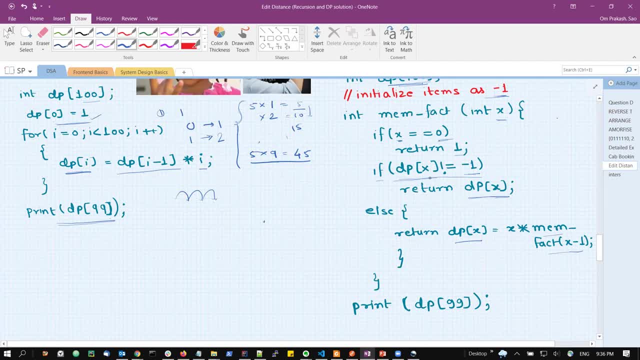 No, Is factorial. a hundred is not equal to minus one. No, it will come here, So initialize factorial hundred as hundred into call the same function for 99.. Again, it will do So. basically it will call for a hundred, So it will make a call to 99.. 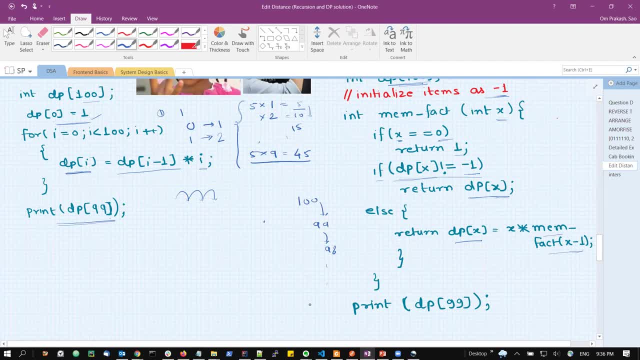 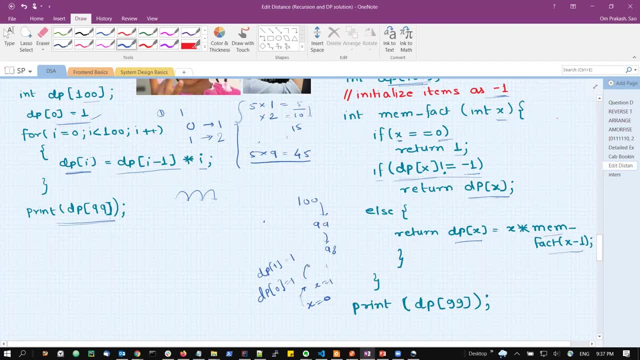 which is the one less than the other. So it will be one into one, which is equal to one, which is equal to one times x, and then it will come up with one to one. So it essentially will keep on going one level up. 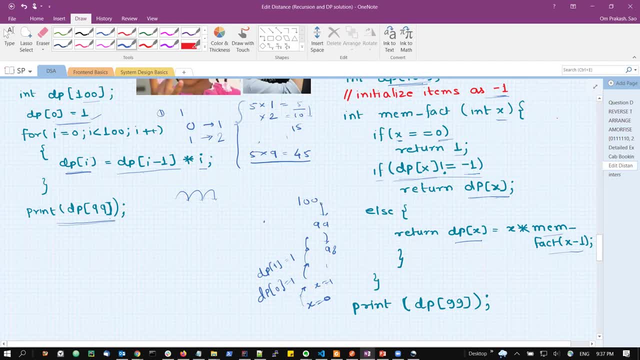 Since one level up for x is equal to one, So dP one is equal to one, x is equal to one times x, one is equal to one into one will be one, And so on. it will keep going one level up. 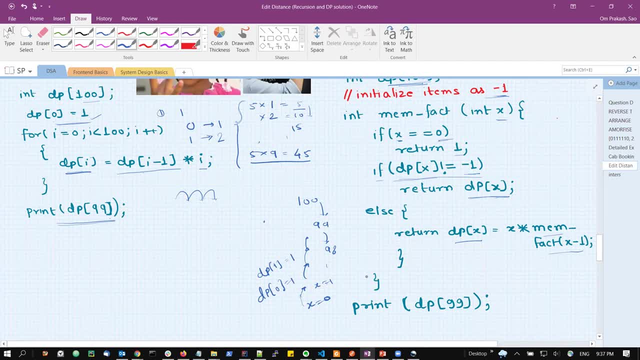 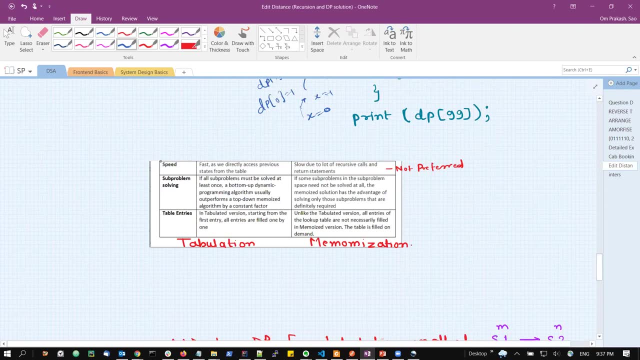 Up, up, up, because you call to initialize all the elements. But initially it has gone from hundred to 99. And to zero, So it is going top. So in terms of the speed, can you just think- or maybe you can pause this video and just think about which one among the tabulation and memoization will be faster? 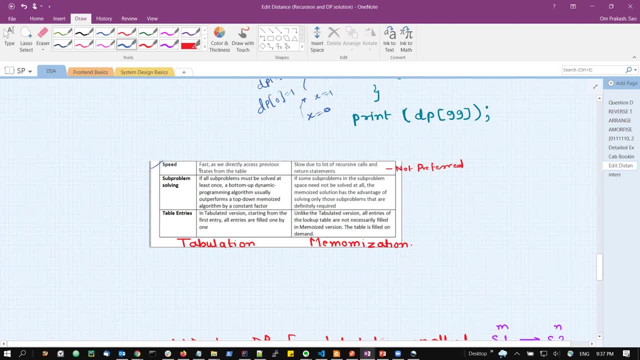 Okay. so because we yeah the tabulation, it will be faster. Why? Because we directly access the previous element. Okay, but in memoization, what is happening? In order to calculate factorial 100, we are going to 99.. 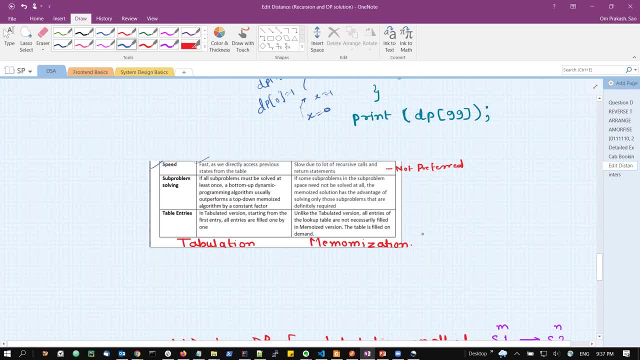 Then we know that, okay, we don't know 99 factorial, So we will go to 98. Oh, we don't know even 98. So basically we are going recursively one level down, down, down, And then we are going up, up, up. So the stack consumption, the stack memory consumption, okay, that will also be very high because lots of recursive calls are being made here. 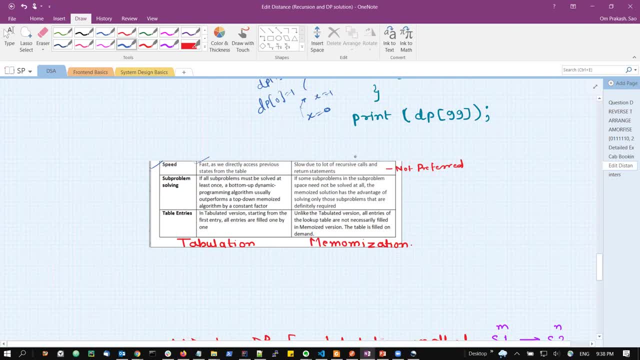 Okay, and also it will be slower. The memoization in this case will be slower If, let us say, we call for the subclass Subproblem solution solving, okay. So if all the subproblems must be solved at least once, if all the subproblems have to be solved at least once, then in that case bottom approach will be better. 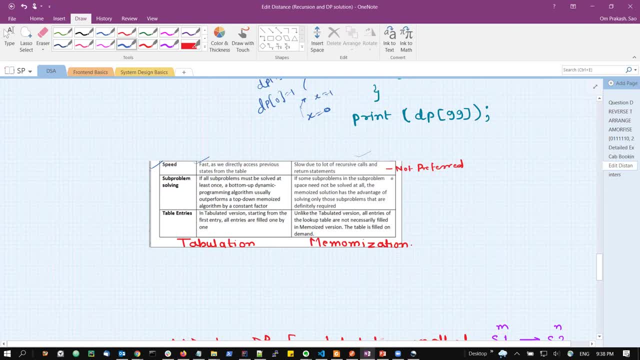 But if all the subproblems are not, they are not needed to be solved- in order to calculate the bigger problem solution. in that case memoization will be better. Why? Because for those sub problems which we are not going to be needing, then there is no point in calculating it, but in 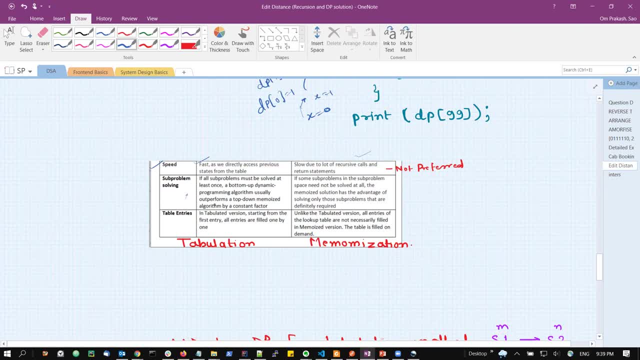 the bottom of approach or in the tabulation approach, they will also be calculated. we are making unnecessary calculation for them also in the bottom of approach, right? so in such case, where all the sub problems are going to be used, tabulation is better. okay, let's come to the